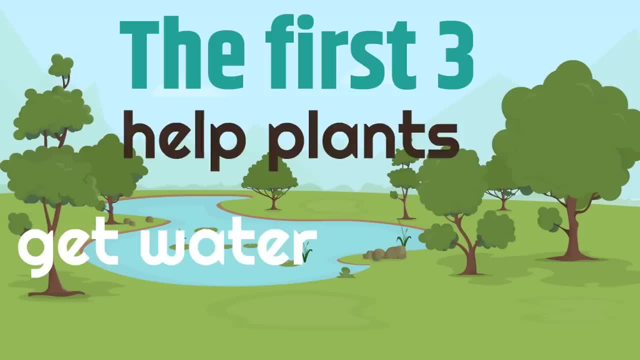 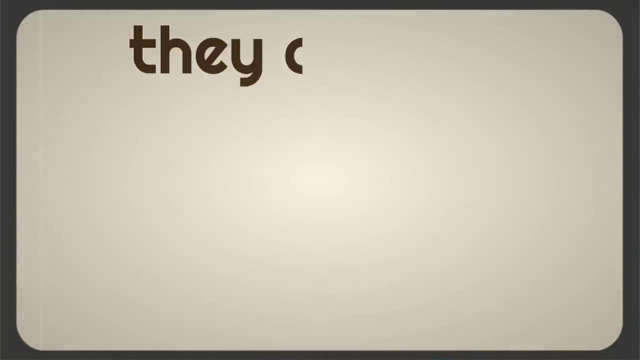 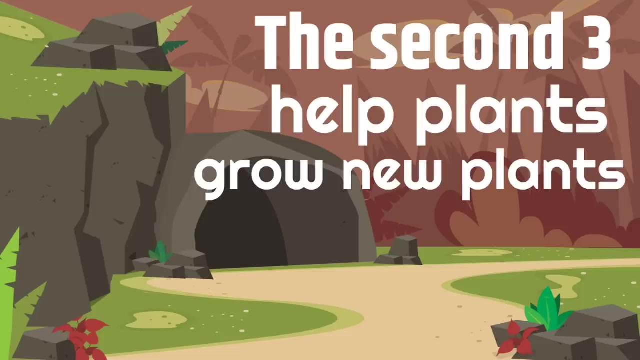 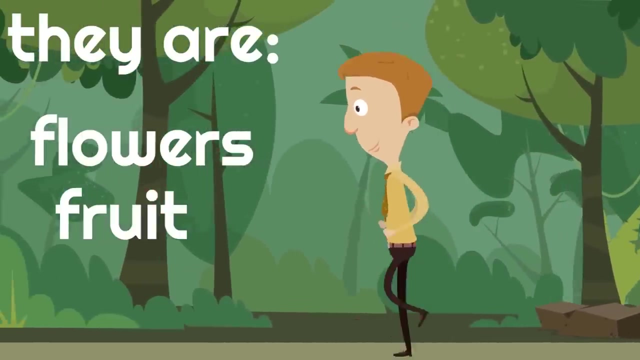 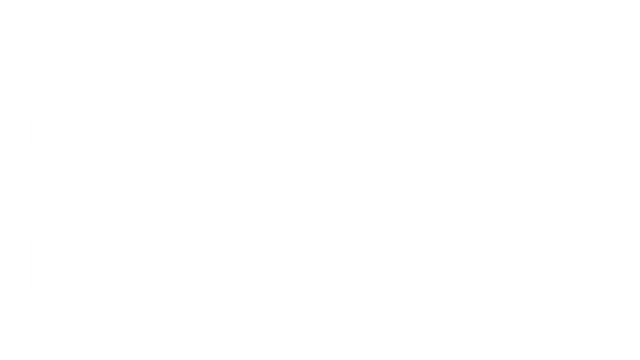 The first three help plants get water, make food and grow. They are roots, stems and leaves. The second three help plants grow new plants. They are flowers, fruit and seeds. So let's learn the plant parts one by one. 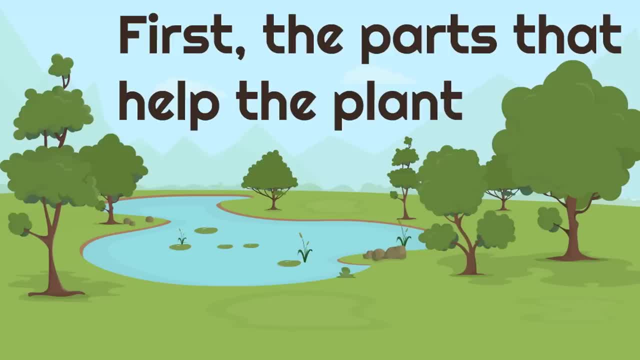 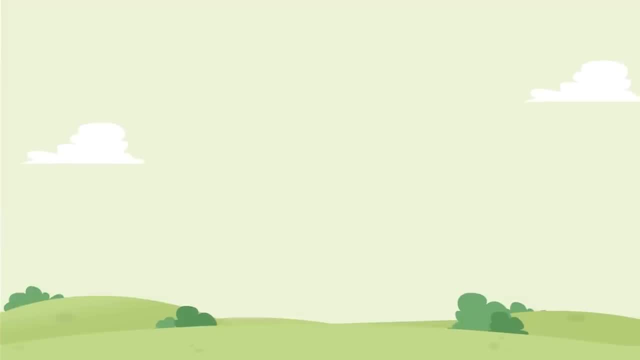 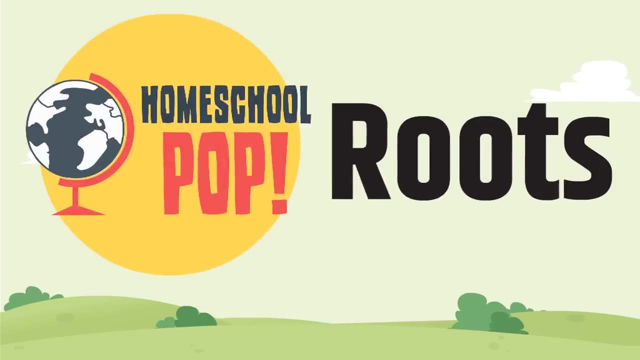 First, the parts that help the plant get water, make food and grow. Okay, so the first plant part we're going to look at today are the roots. Roots have a special job. You see, roots hold the plant in the soil. 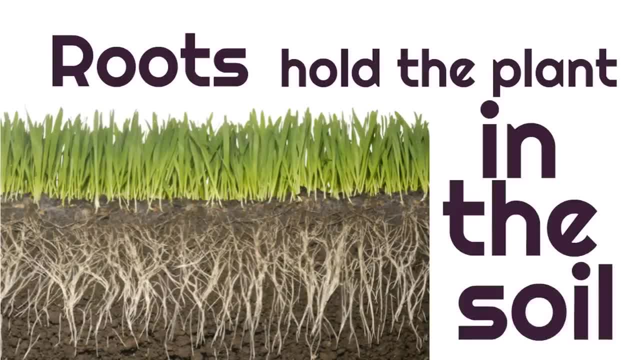 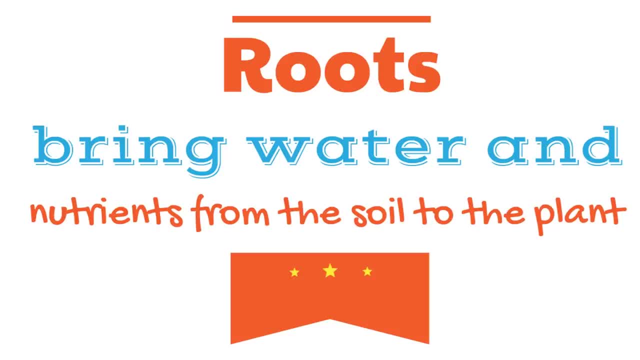 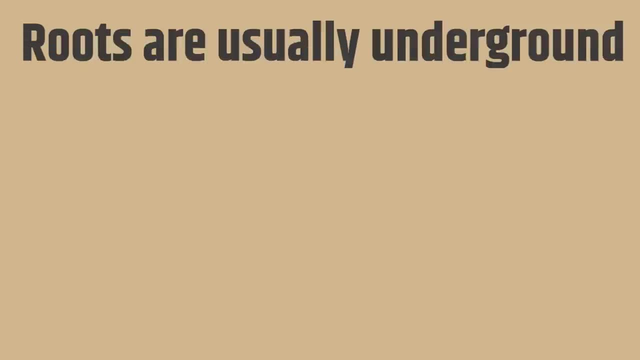 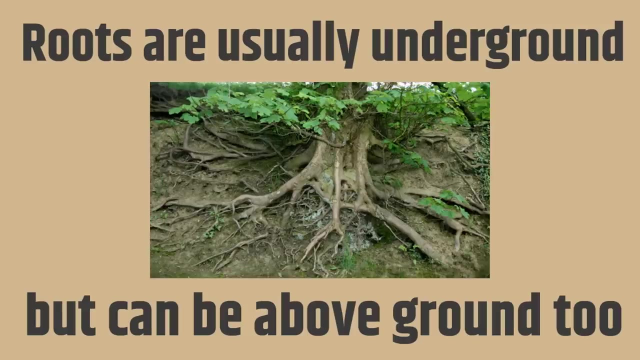 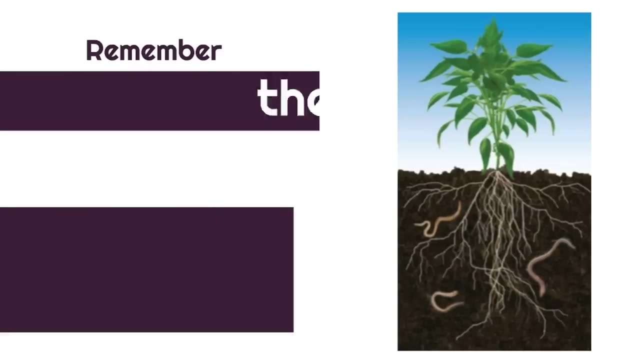 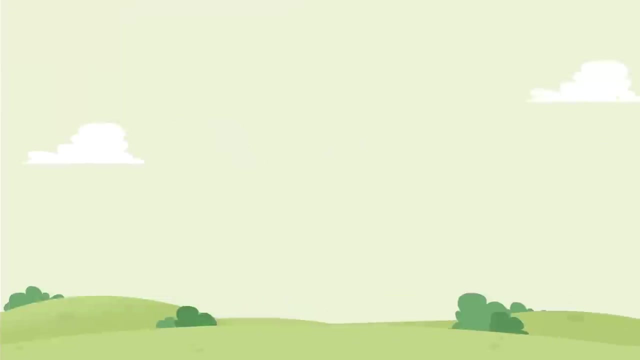 The soil is the dirt in the ground. Then roots bring water and nutrients from the soil to the plant. Roots are usually underground, but can be above ground too. Have you ever seen a tree that looks like this, where the roots are above ground? Remember, the roots hold the plant to the soil. 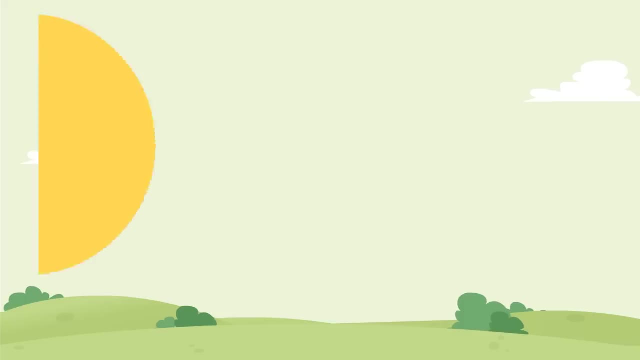 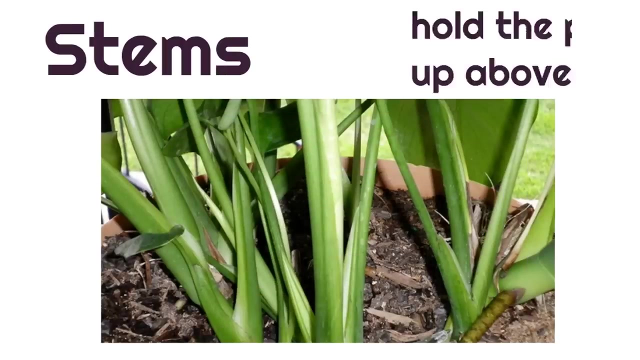 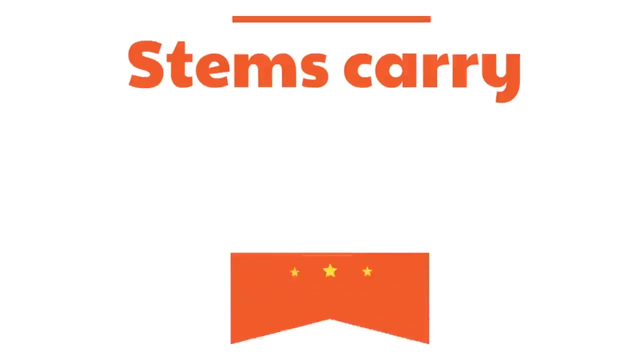 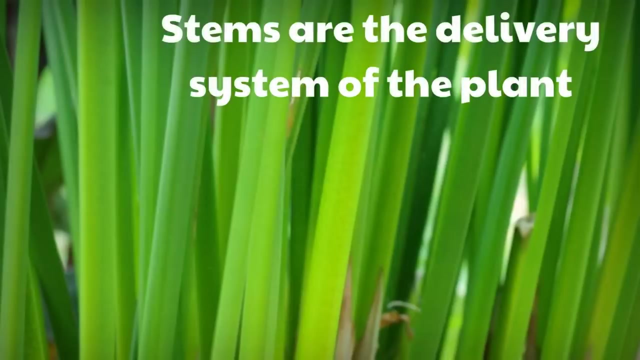 Okay, so now we're going to look at the second part of a plant, which are the stems. Now, the stems hold the plant up above ground. The stems carry water and food through the plant. Stems are the delivery system of the plant. Roots get water and nutrients from the soil. 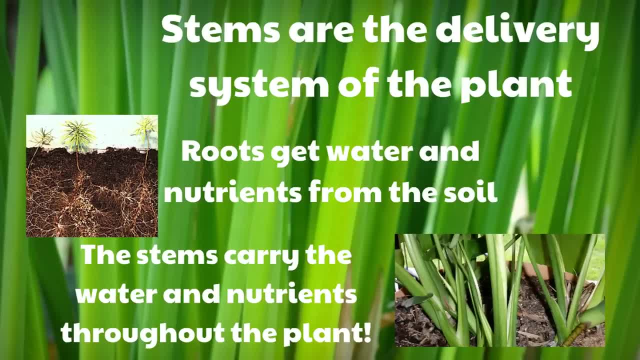 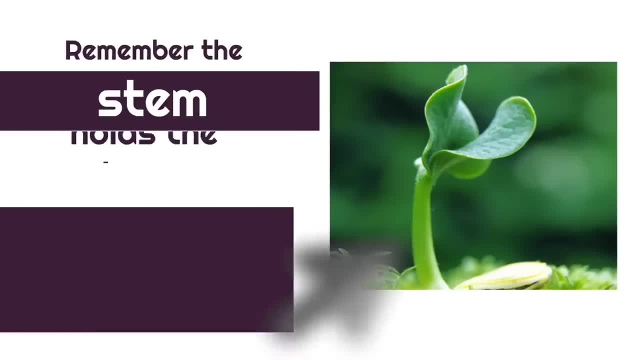 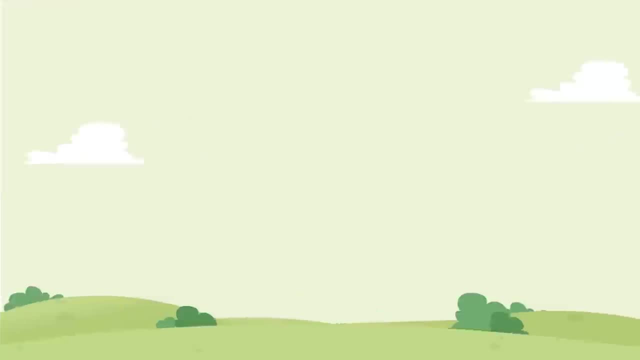 And the stems carry the water and nutrients from the soil between the roots and the plants throughout the plant. Remember, the stem holds the plant above ground. The next part of the plant we're going to learn today are leaves. The leaves are on the 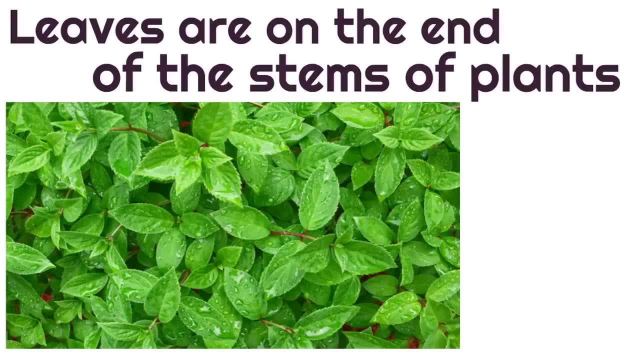 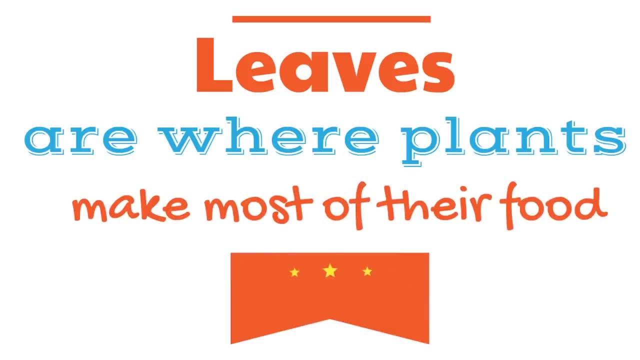 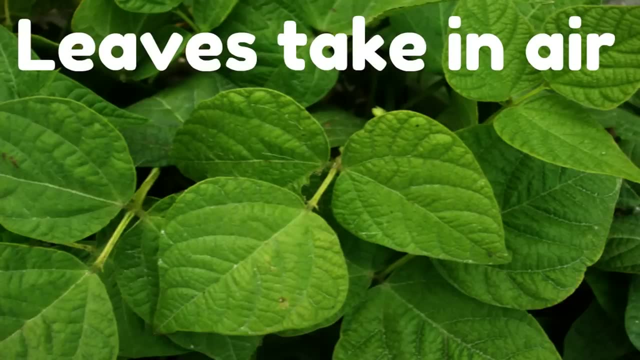 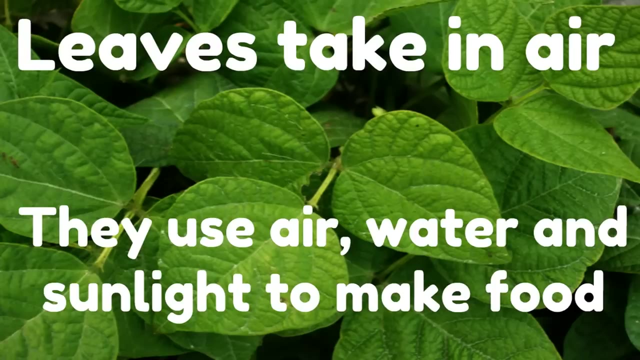 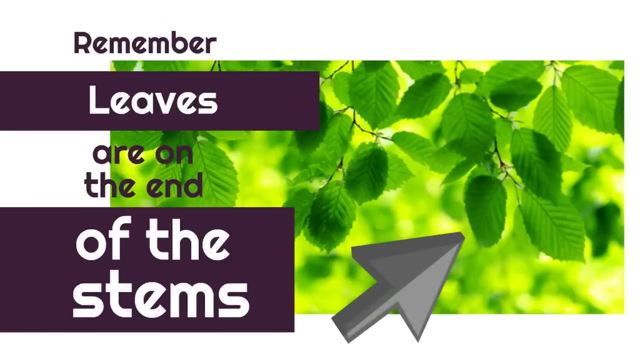 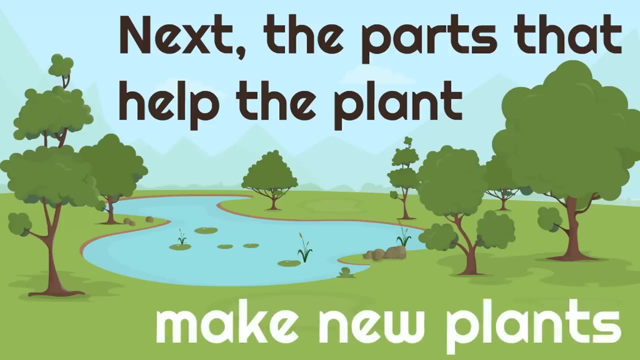 end of the stems of plants, And this is interesting. Leaves are where plants make most of their food. Leaves take in air and they use air, water and sunlight to make food. Remember, leaves are on the end of the stem. Okay, so next the parts that help the plant make new plants. 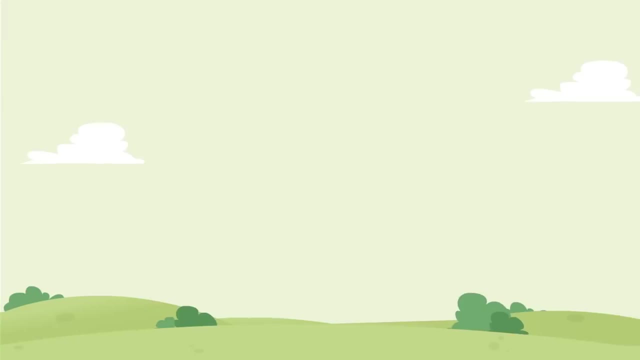 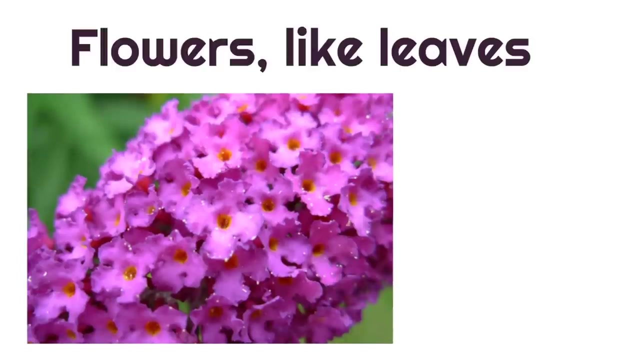 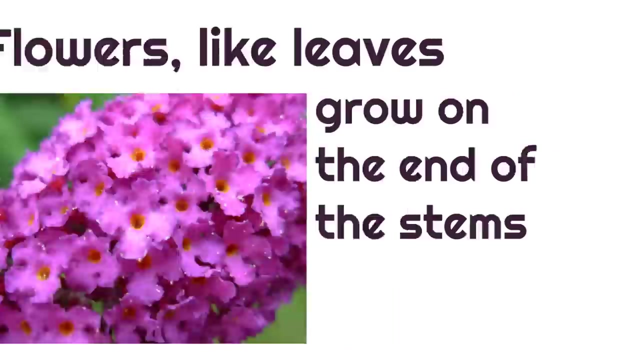 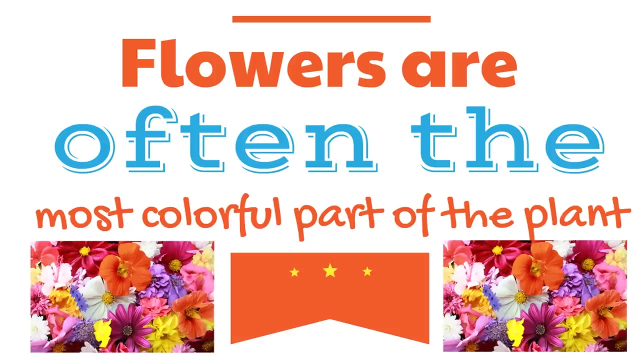 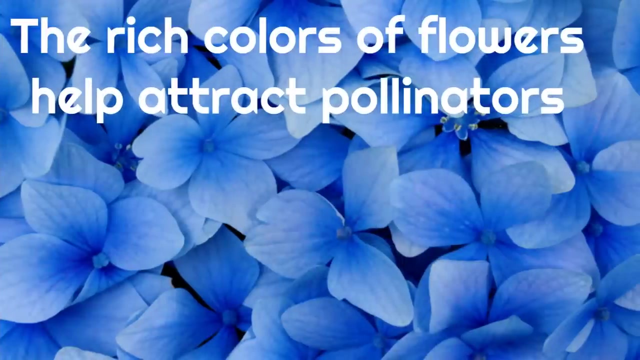 The next part we're going to look at are flowers. Flowers, like leaves, grow on the end of the stems. Flowers are often the most colorful part of the plant. Okay, now, this is awesome. The rich colors of flowers help attract pollinators. 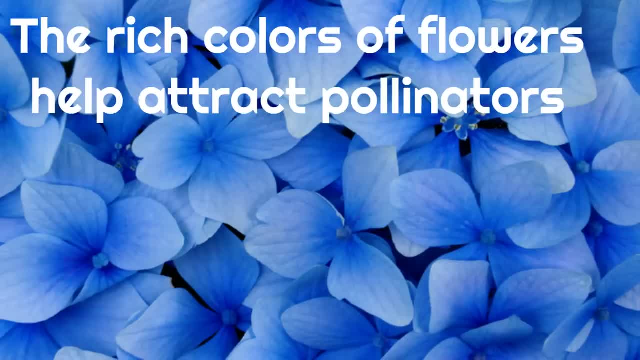 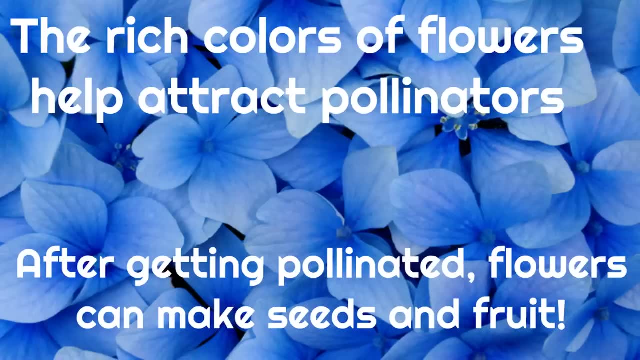 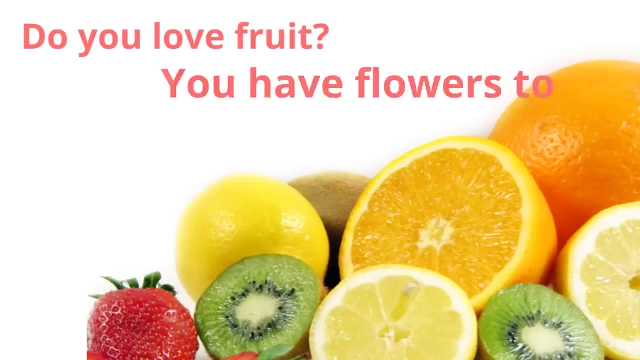 That's why they're beautiful. The beauty has a purpose. After getting pollinated, flowers can make seeds and fruit. Do you love fruit? Yes, fruit is awesome. You have flowers to thank for that. Flowers make fruit. So the next time you're eating an amazing piece of fruit, just think to yourself. thank you flowers, Thank you flowers. 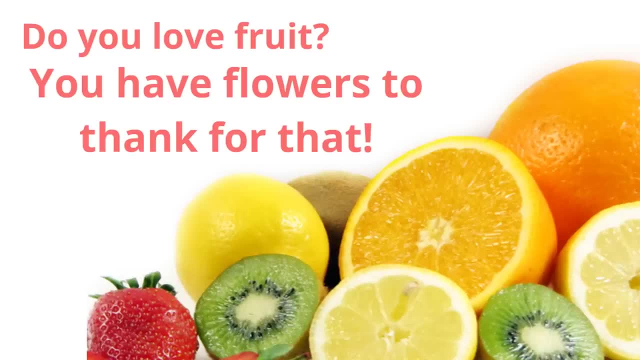 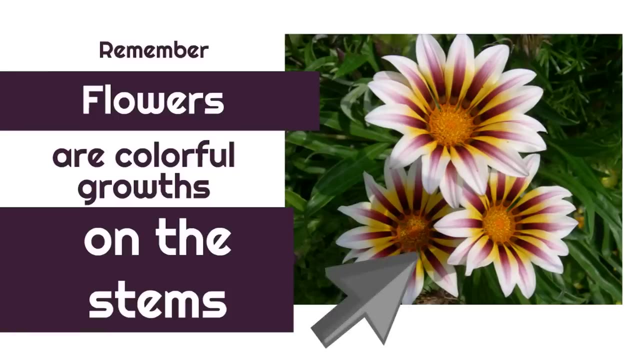 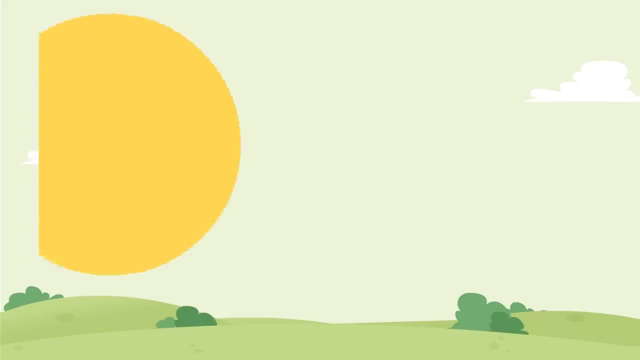 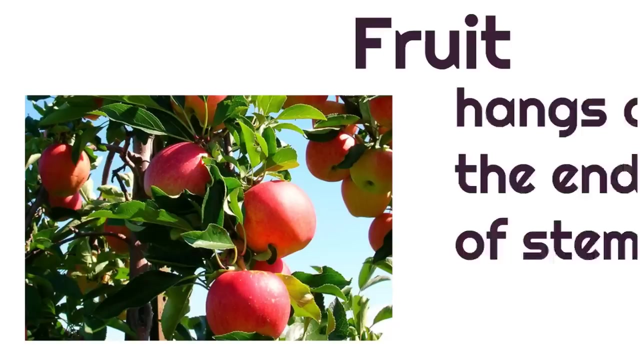 Remember, flowers are the colorful growths on the stems. The next part of the plant we're going to learn about is the fruit. Alright, now, where on the plant is the fruit? Fruit hangs on the end of stems. Now you might be wondering: what's the fruit's job? What does the fruit do? 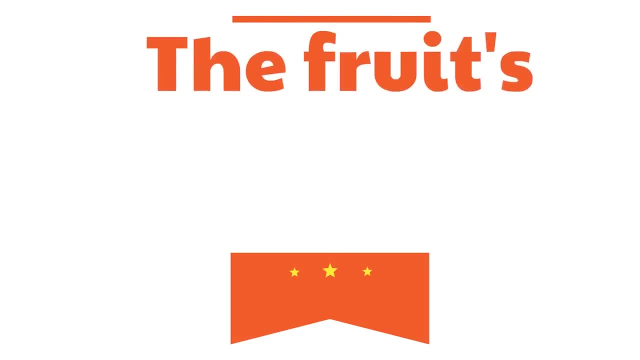 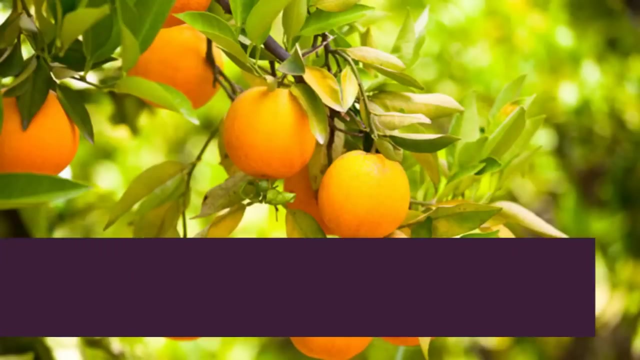 Well, the fruit's job is to hold the seeds. The fruit needs to be held by itself. The flower needs to be held. Fruit is just a delicious seed holder. Now, either one of two things happens to fruit: Fruit is either picked and eaten, or it falls off the plant and rots. 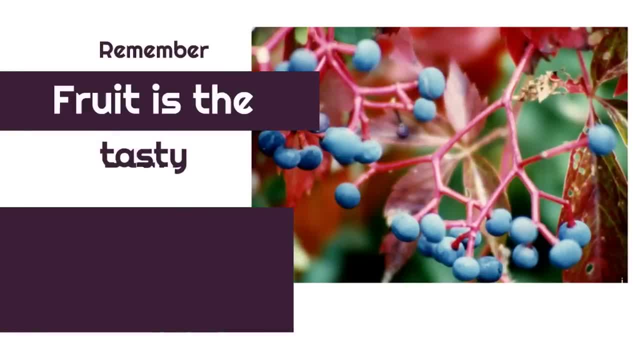 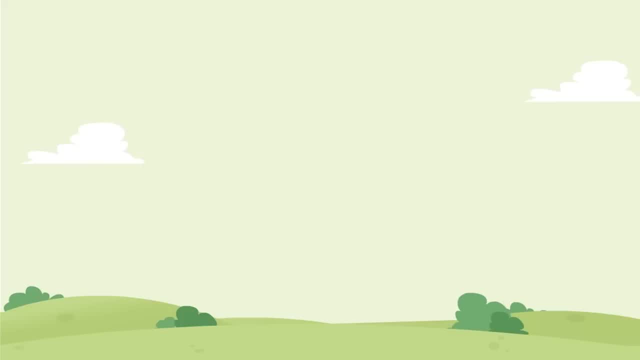 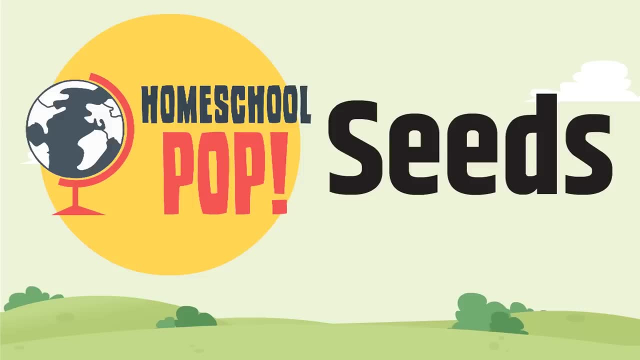 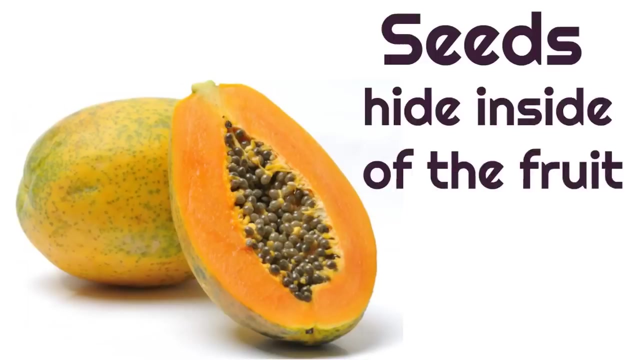 Remember, fruit is the tasty stuff on the stems. Okay, the last part of the plant that we're going to learn today are the seeds. So where are the seeds of the plant? Seeds hide inside of the fruit. Now, the seeds have an incredible job. 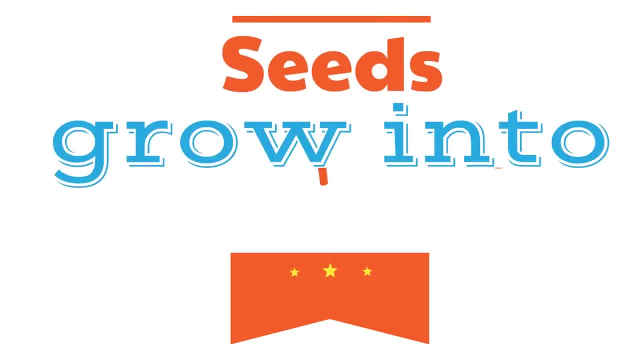 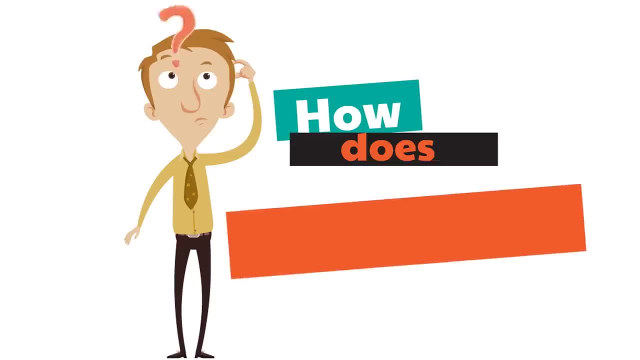 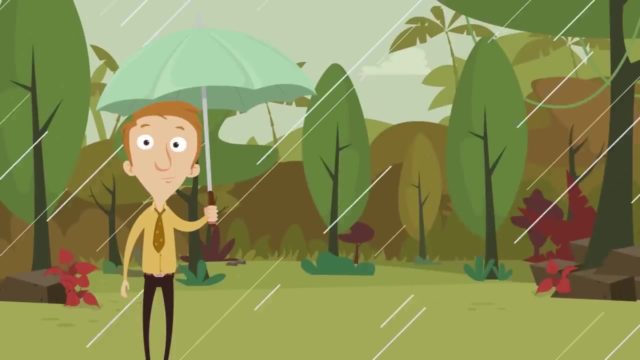 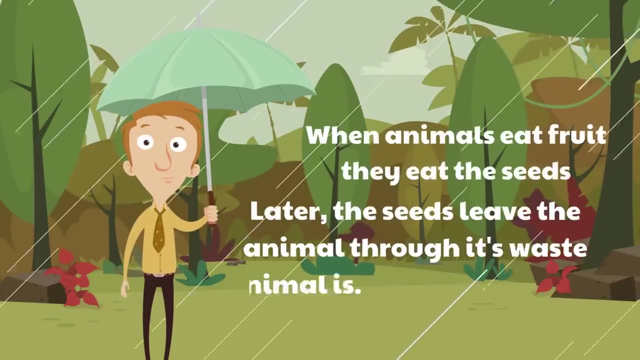 You see, seeds grow into fruit And they grow into new plants. Okay, you might be wondering: well, how does that work? Well, here's one way: When animals eat fruit, they eat the seeds. Later, the seeds leave the animal through its waste, wherever the animal is. 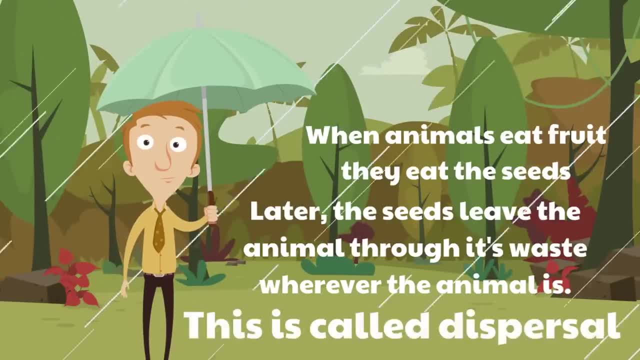 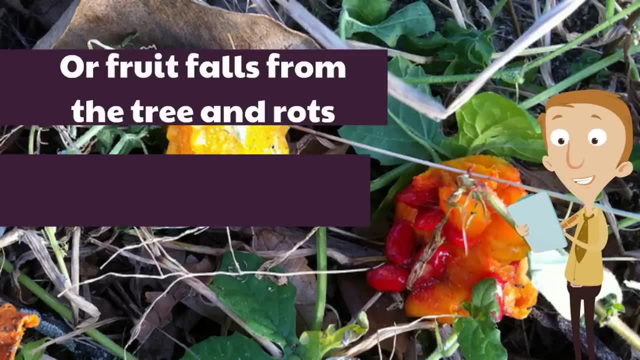 This is called dispersal, Or fruit falls from the tree and rots. The word rots means dies. The fruit dies, It rots, The seeds fall out and can make a new plant. The first way, called dispersal, takes the seed to another place, so it plants a new plant in a new place. 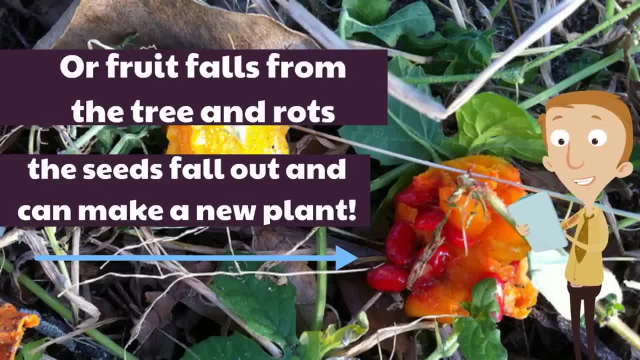 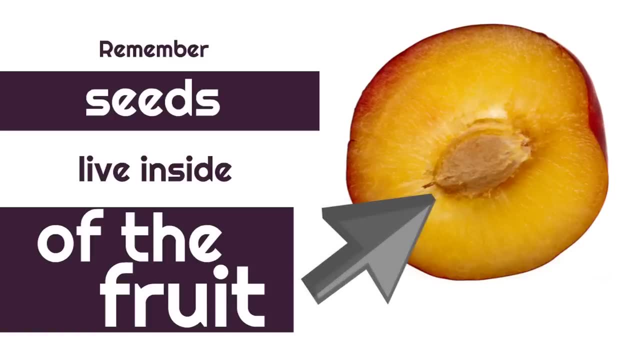 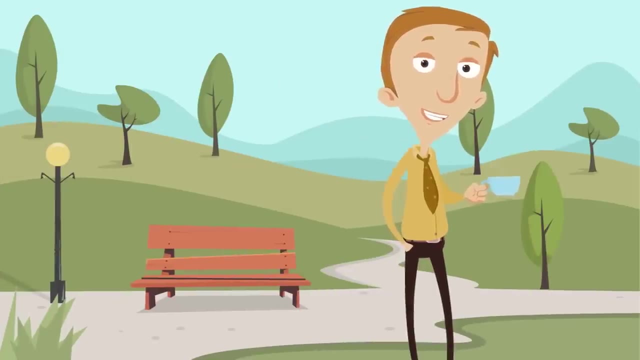 When a fruit falls and rots, it plants a new plant nearby the original plant. Remember, seeds live inside of the fruit. Hey, it looked like you were doing a good job paying attention, learning about the plant parts, And now we want to see how much you learned. 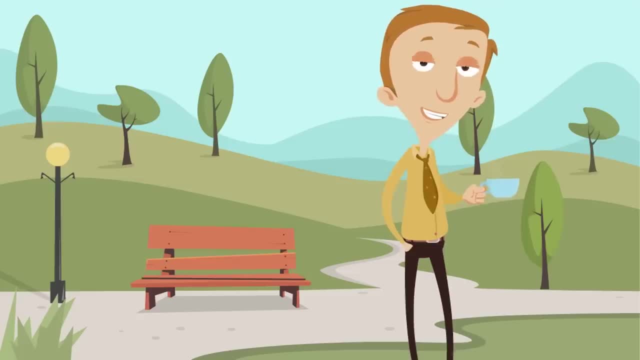 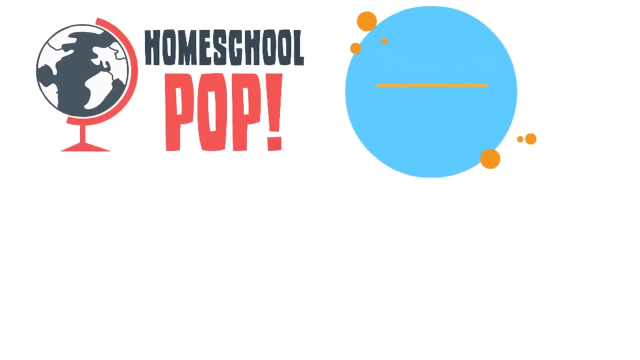 We're going to play a game called name the plant part. We're going to show you a plant part And then you go ahead and tell us which plant part it is. Alright, hope you're ready, because here we go. Look at this picture of a plant.